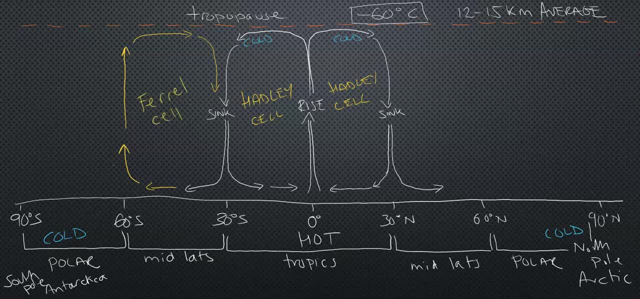 called the ferrule cell. that's next to the Hadley cell. So we can do the same thing over here on the northern hemisphere. The wind approaches 60 north. It's going to rise up. It's going to rise up towards the pores, It's going to split. and it's going to split over here in the southern hemisphere. 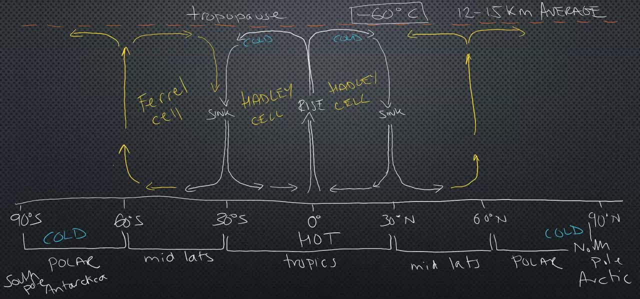 as well and it's going to rejoin the Hadley cell here at 30 degrees north and sink because it's very cold and we have our ferrule cell over here. So we have our symmetrical cells forming because of air that's either being heated and rising or it's cold with less heat and it's going to sink. 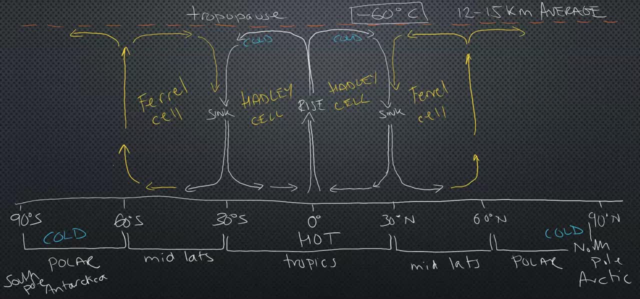 and there's a final cell between 60 south and 60 north and 90 north and 90 south, and this is the polar cell. So we're going to have this situation where the air is going to sink again. It's very, very cold and it's going to sink down towards or over 90 south. It's going to come back around. 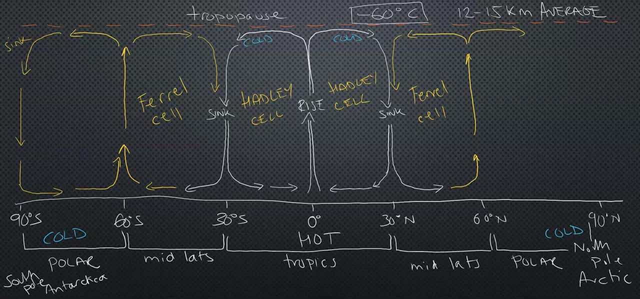 across the surface as wind and rejoin at 60 and rise up. So we're going to have this situation where it's going to rise up. So we have a rise in section right here over 60 and it's going to sink down. It's very cold air. It's going to sink over 90 south, which is the south pole, Antarctica, and 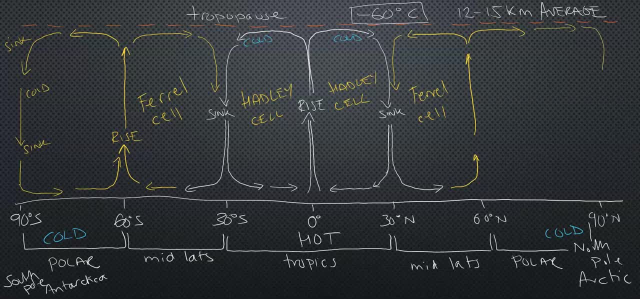 the same thing is going to happen over here in the northern hemisphere. So it's going to sink down very cold over 90 north. It's going to sink and it's going to hit the surface and be pushed back and rejoin at 60 north, which is going to rise up and we have our polar cell in the northern. 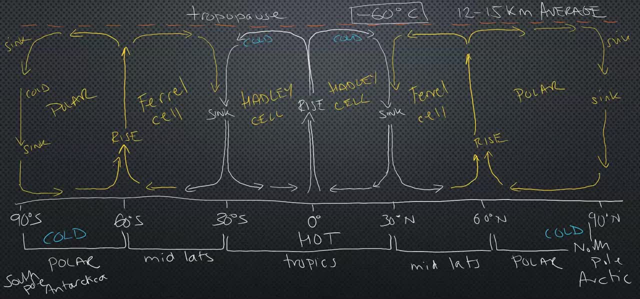 hemisphere, Polar cell in the southern hemisphere. So again we have a symmetrical set of three cells: Hadley, Ferrell, Polar. So the simple heating and cooling of air in the troposphere from the equator, because the equator is heated more than the poles. 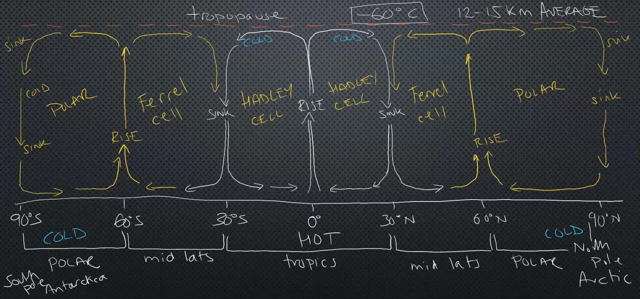 and you have this differential heating. You have these three symmetrical convective cells that form in the troposphere called the Hadley, which is around the equator, the Ferrell in the mid latitudes, and the Polar, Obviously the polar regions that form to move heat and that requires air. It's going to carry the heat.